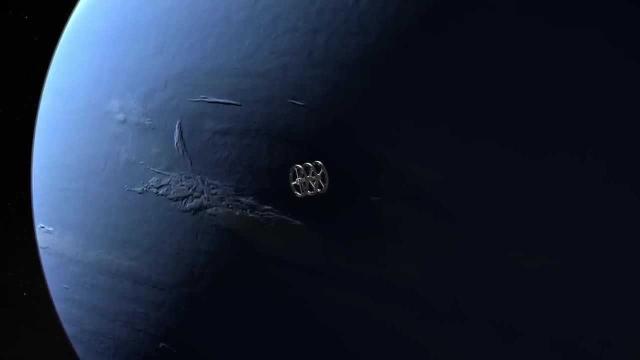 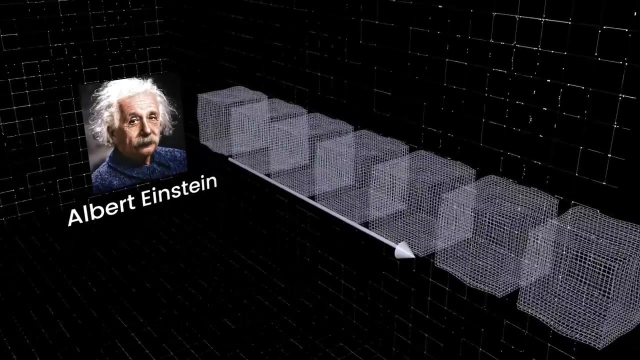 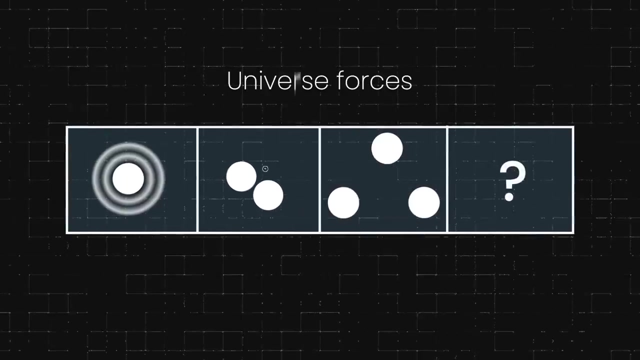 tiny scale, But these two theories don't work well together and they often contradict each other. Albert Einstein managed to unify space, time and gravity, But the other forces of nature were missing. to finally connect all these under one framework, Unlike other forces in the universe. 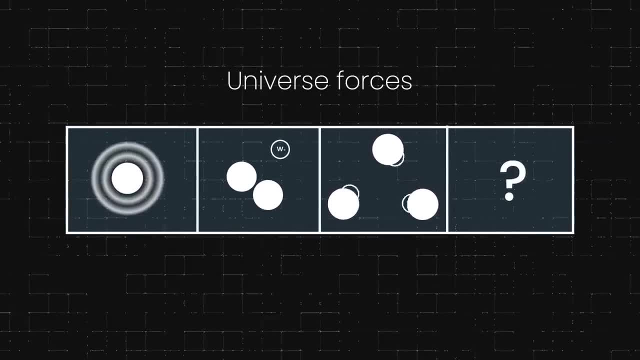 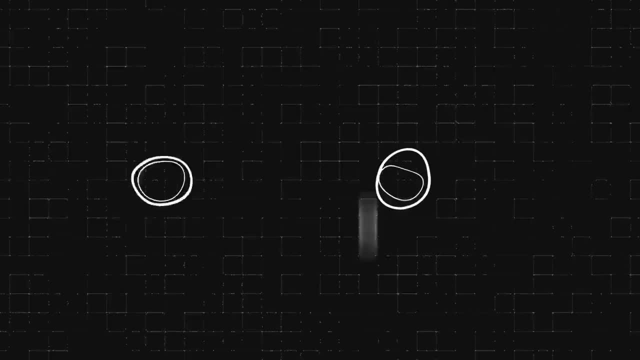 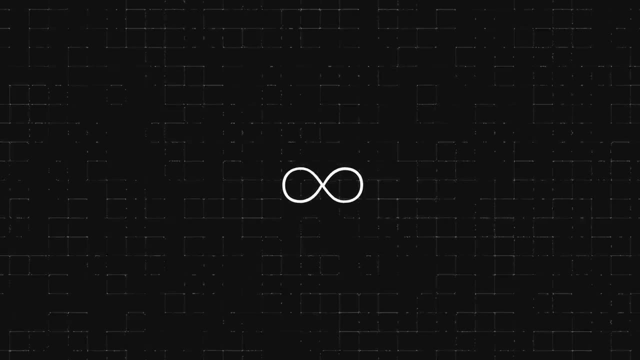 What a particle called a graviton should look like. But once they try to predict what happens when gravitons collide, they get an infinite amount of energy packed into a very small space, And this means mathematics is missing, something We only know: gravity exists because of its effects. 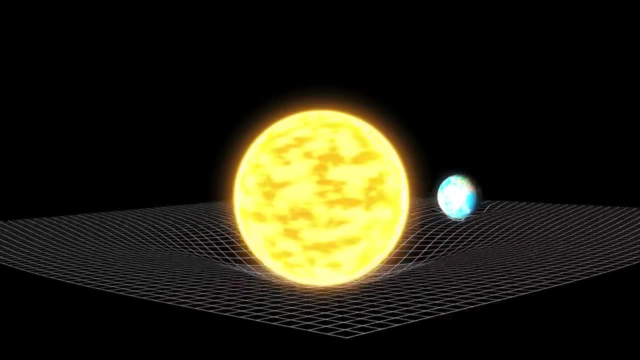 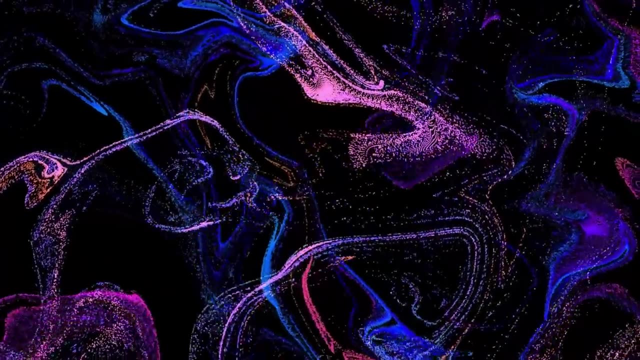 only noticeable and important on the scale of extremely large objects in space, But quantum particles are so tiny gravity becomes irrelevant in their interactions. String theory was born in an attempt to connect both these two forces of gravity, And this is why we have a very small space. 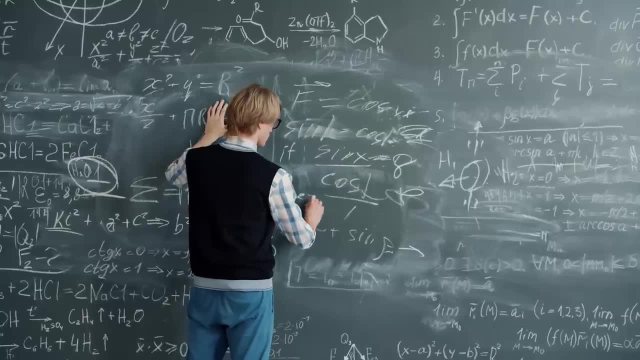 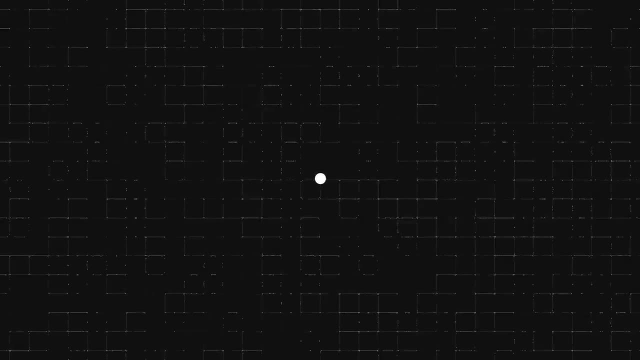 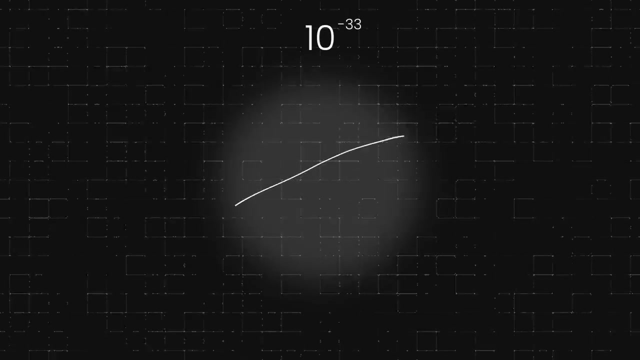 And so what is this theory? It suggests that a particle isn't a point-like object, but rather a one-dimensional strand of energy or a string smaller than an electron or quark, or about 10 to the minus 33 centimeters. 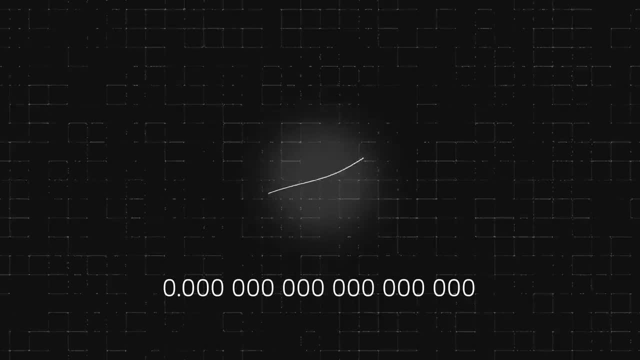 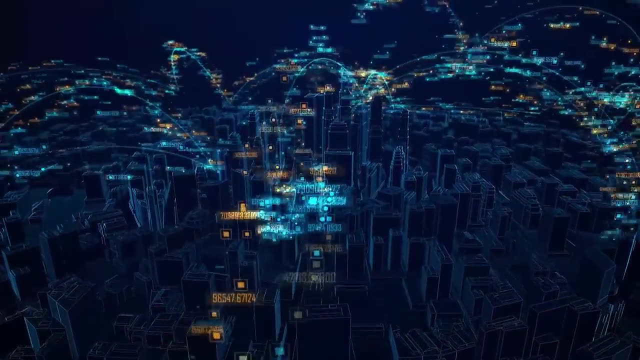 in length, which is a millionth of a billionth of a billionth of a billionth of a centimeter. But while things that we see can move left or right, up or down and back or fourth, strings can move in at least ten different ways and be either open or closed, And some 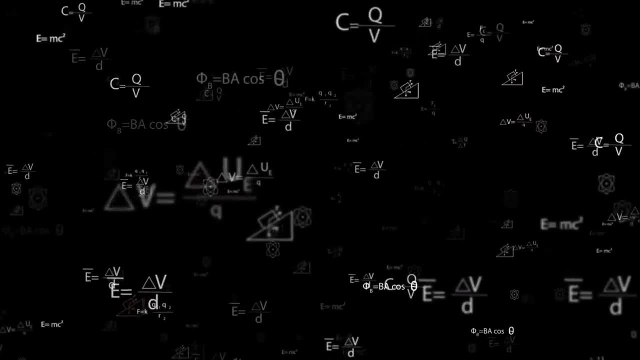 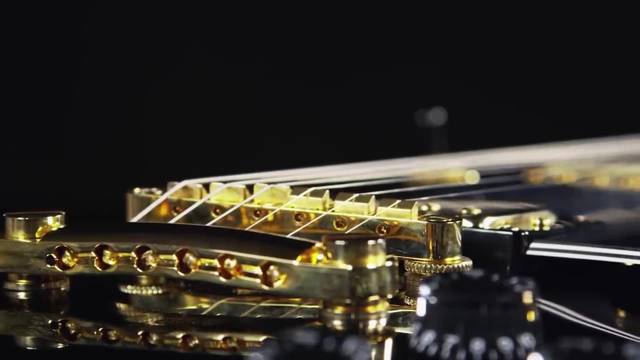 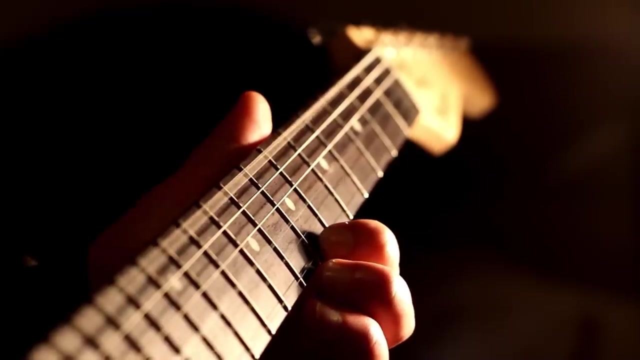 physicists think that the way strings move determines the attributes of all the things in the universe. To understand how strings can obtain properties of particles, imagine a guitar. Its strings are one-dimensional, but they can move in three dimensions when pulled, and the way they move determines the sound they make. In a similar way, quantum strings twist. 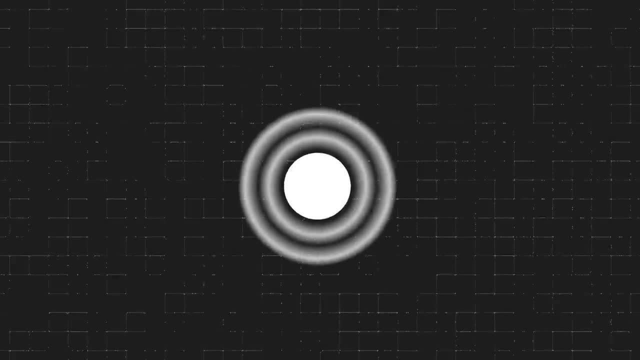 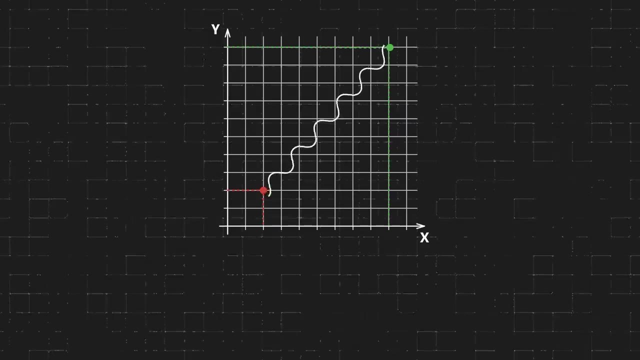 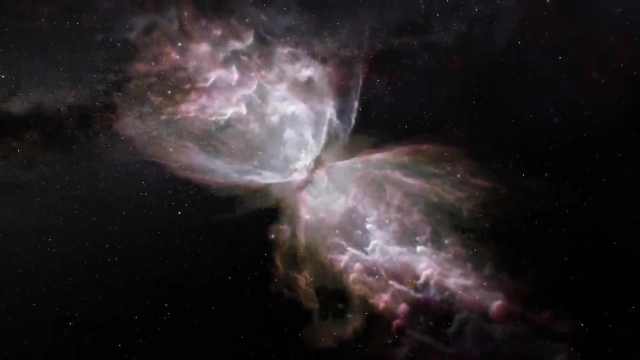 and turn or vibrate at different frequencies, which then creates the forces in our universe. This is also how a one-dimensional string of a certain length can twist. in a way, it would appear to us as a photon, a quark or even a graviton. Now, physics is largely based on 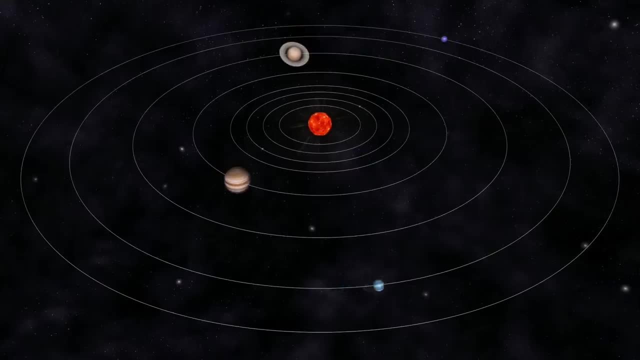 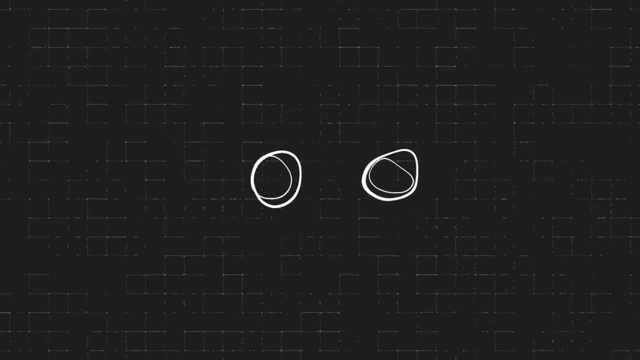 mathematics and scientists often reach a dead end trying to explain or calculate things, just like with gravity. But if you replace point-like gravitons with strings, mathematically they can collide and move in the same direction And that's why we call them gravitons. 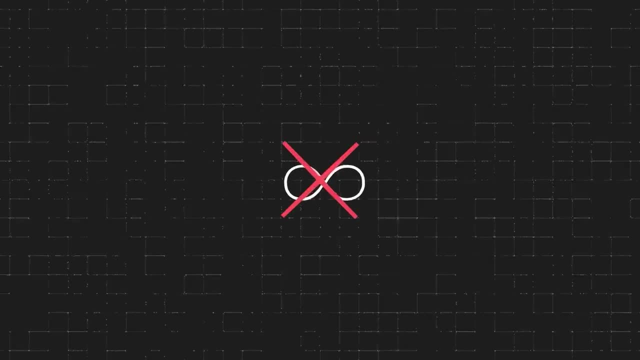 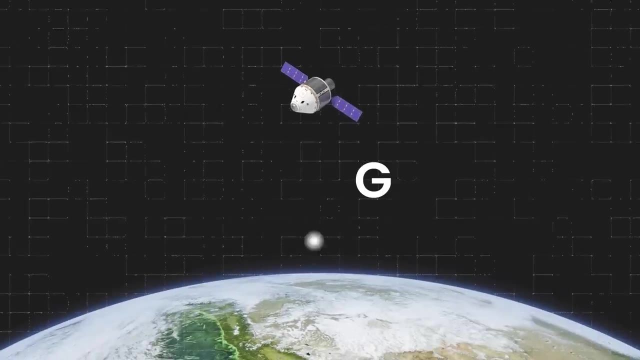 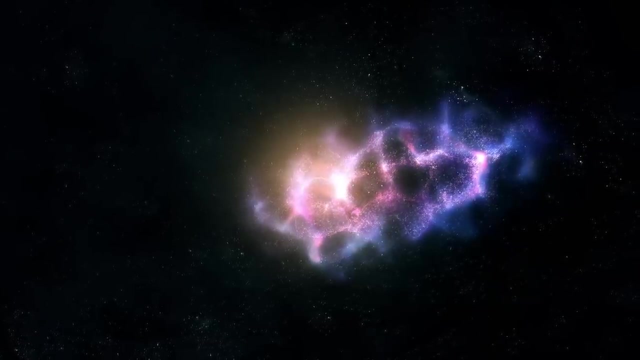 String theory predicts the existence of the gravity particle, helps us calculate its interactions with other particles, and so can describe quantum gravity. Scientists have used string theory to explain different phenomena, such as the creation of the universe, dark energy or what's happening. 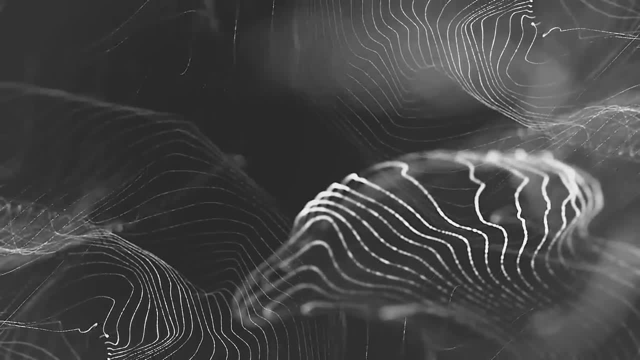 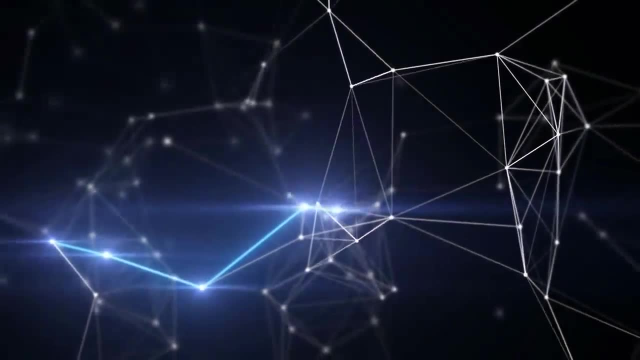 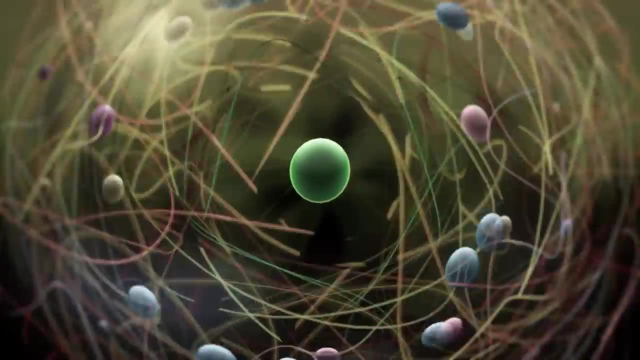 inside black holes. The theory even implies the existence of hypothetical particles such as axions, in an attempt to explain dark matter and many more additional particles. There's a lot of potential in string theory, but there are problems with it too. With current 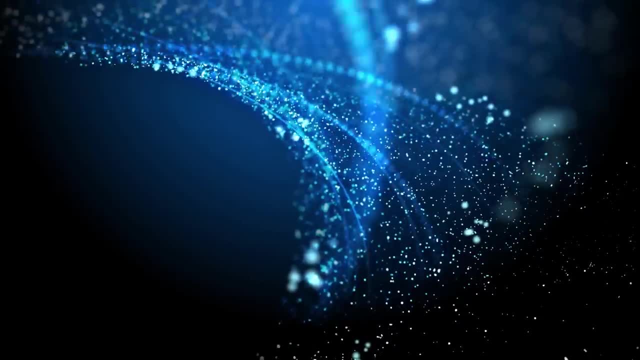 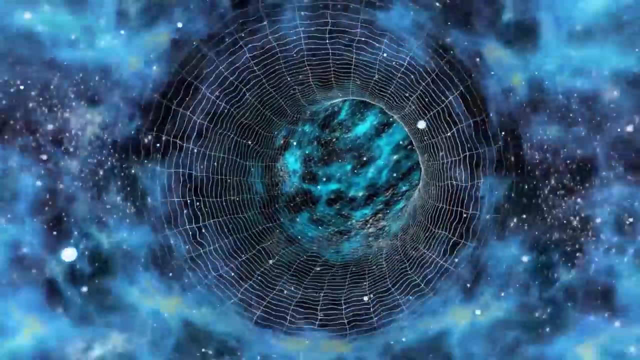 technology we can't prove if its predictions are correct. While some physicists believe string theory is our best chance to combine quantum physics and gravity, others say it's pseudoscience, as it seems to be almost impossible to test through experiments. And then there are dimensions. 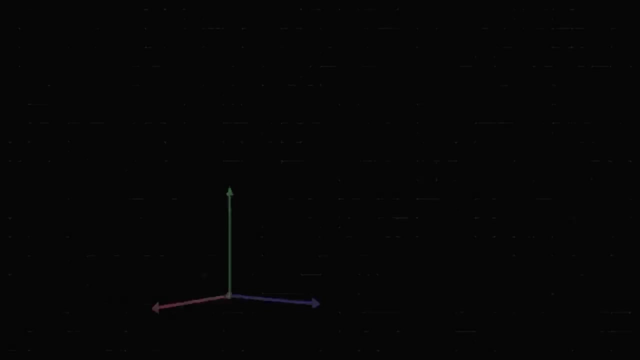 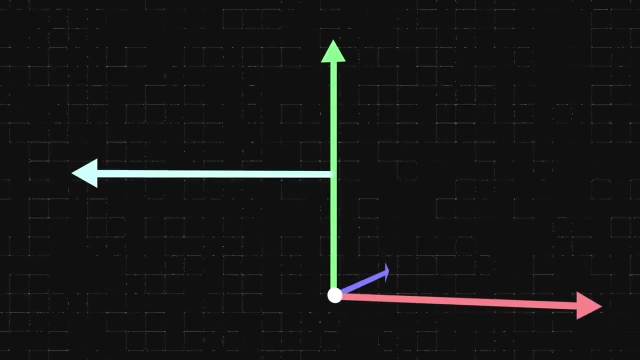 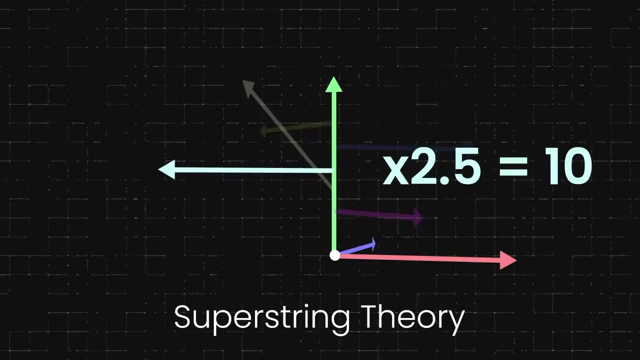 Dimensions. We think our universe consists of three dimensions of space and one dimension of time. But for string theory to work we have to assume there are 26 dimensions, although a more complete superstring theory cuts down the dimensions from 26 to 10.. But even then there are three dimensions of space and one of time. 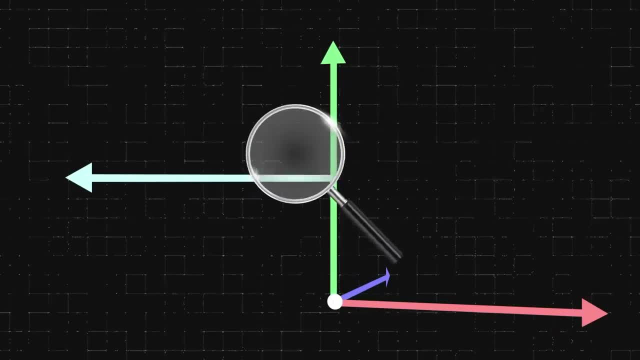 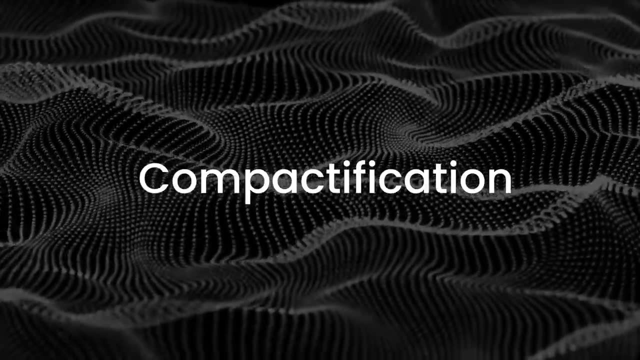 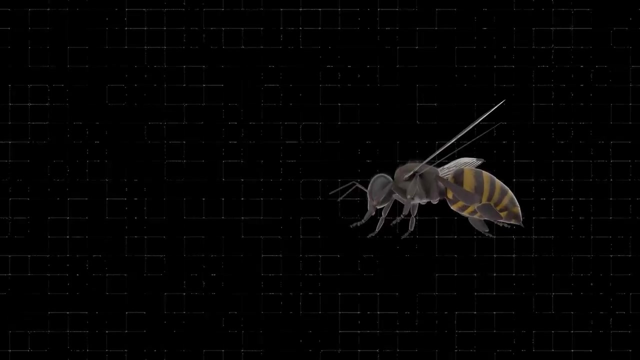 So if these six additional hidden dimensions exist, where should we look for them? One idea is that they are undetectable to us because of the process called compactification, meaning these dimensions are tightly curled up on themselves. Imagine a power line To a bee flying far above it. 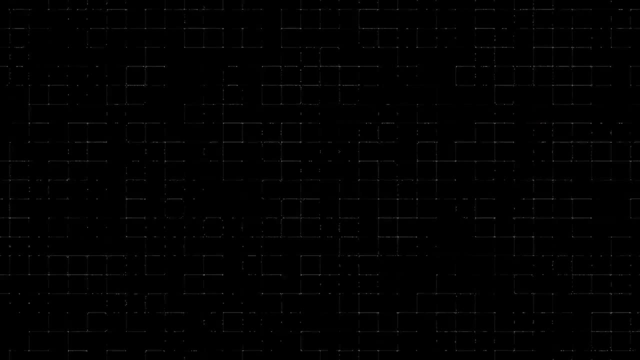 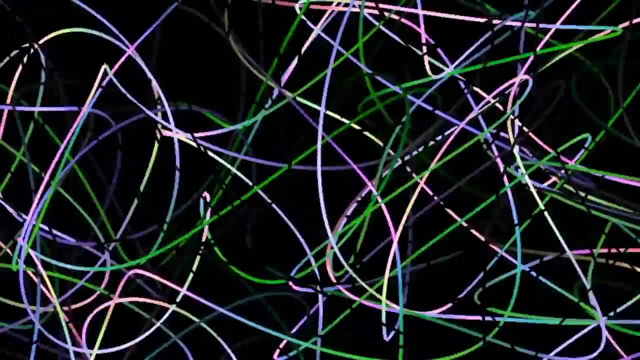 it would appear as a 1D line, But to an ant crawling on top of it, this same line would be a 3D cylinder. According to string theory, something similar can be happening to dimensions in our universe. The possibility of these additional dimensions would also increase. 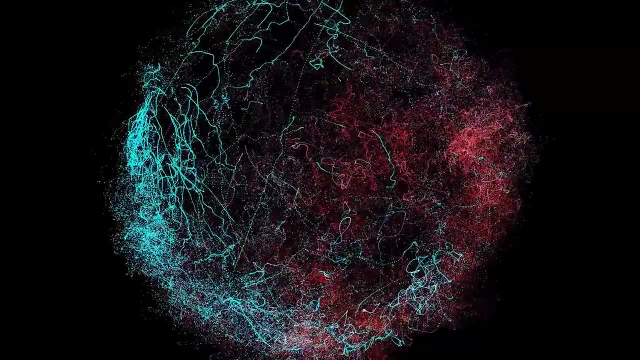 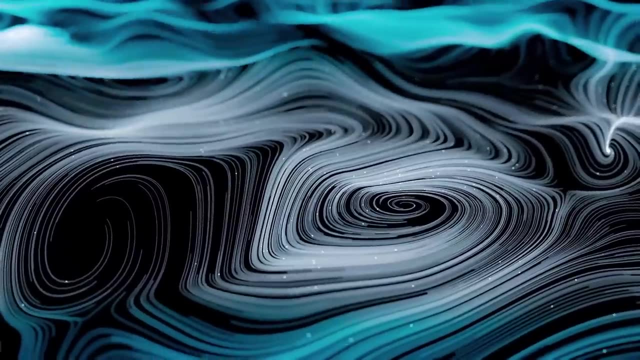 the number of frequencies in which strings could vibrate, which would mean a bigger diversity of particles. There are many ways in which six dimensions can be curled up. Every combination would result in a different spacetime or a different universe filled with different particles. 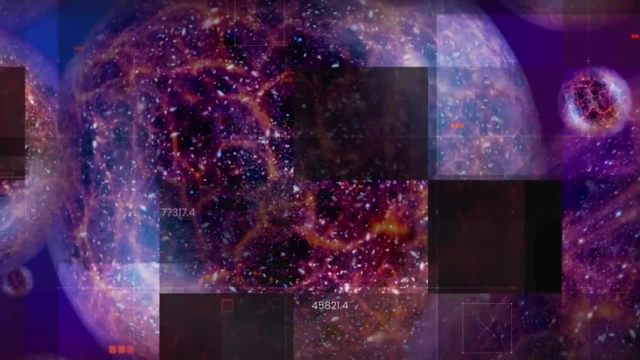 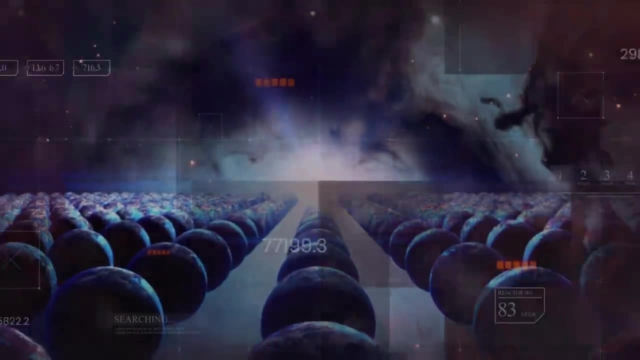 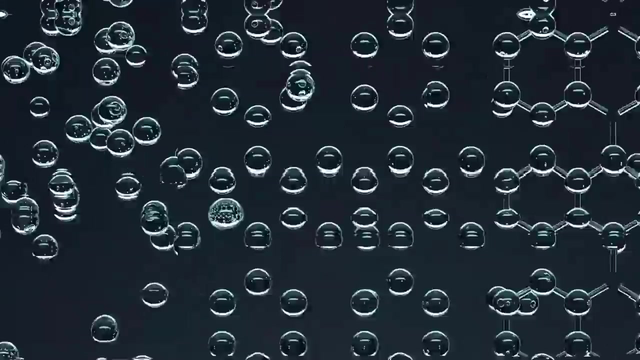 So string theory also implies there's a multiverse of universes, A tremendous number of one followed by 500 zeros. Because of this, there are a quadrillion ways. an exact version of our universe, with the same set of matter, particles and fundamental forces could be made Among a. 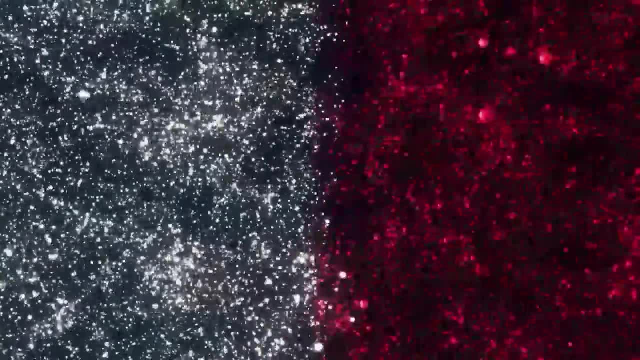 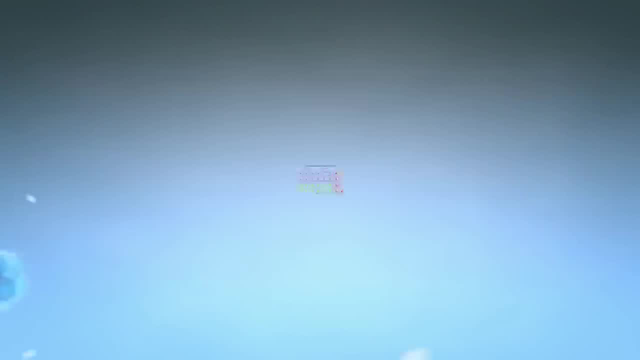 huge variety of possibilities. there are many ways in which a multiverse of universes could be made. However, we don't know why our universe would have the particles of the standard model instead of some other particles. There are hypotheses suggesting the geometry of our universe might. 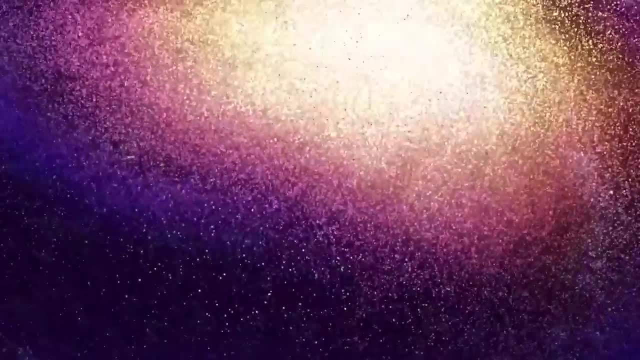 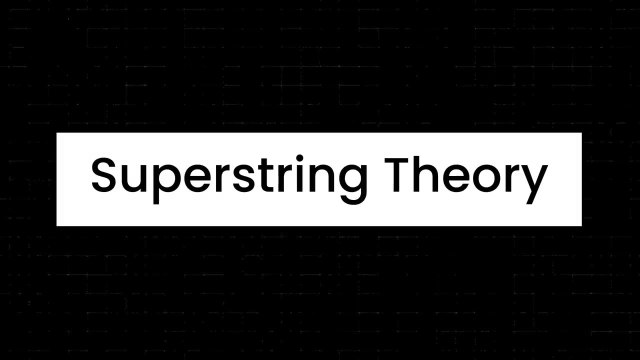 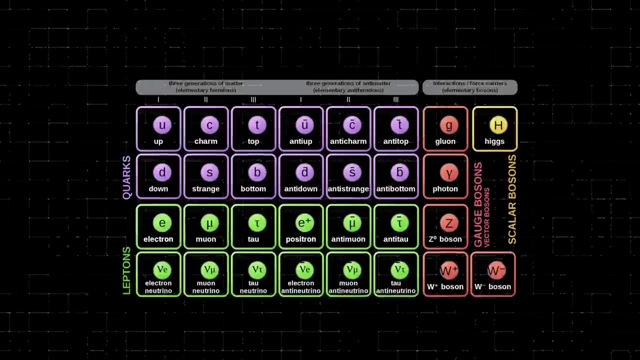 have changed over time, transitioning from one compactification to another, And if so, the laws of physics would have changed too. According to superstring theory, particles in the standard model have supersymmetric partners, And we have already once predicted the existence of electrons, positrons and others. 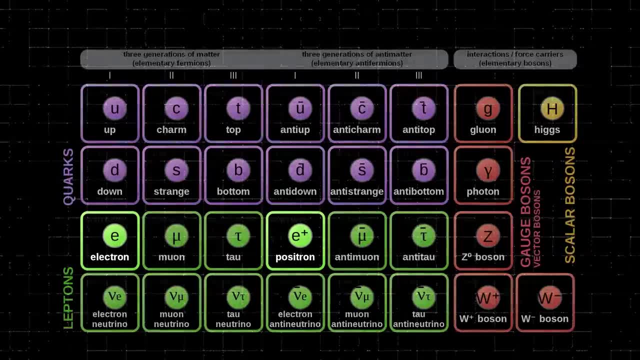 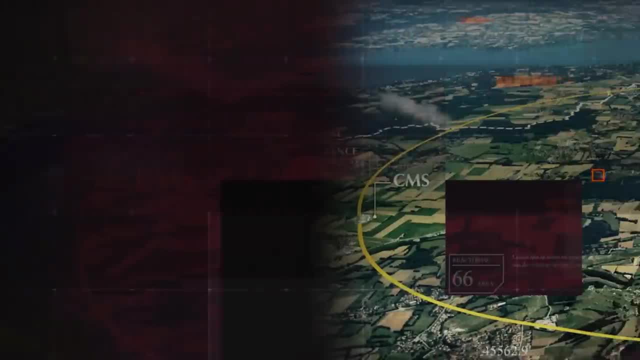 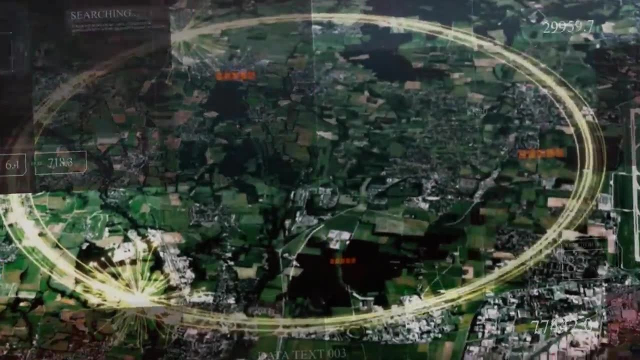 But if these superpartners exist, we'll have to build a much bigger version of the Large Hadron Collider that would create collisions about 7 million times more energetic to test the idea. There have been many variations and upgrades of string theory, and there's even a unified 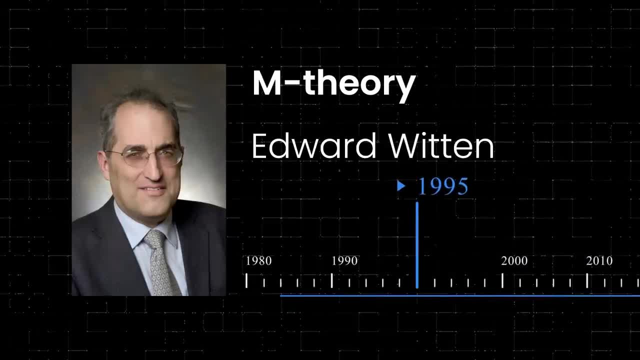 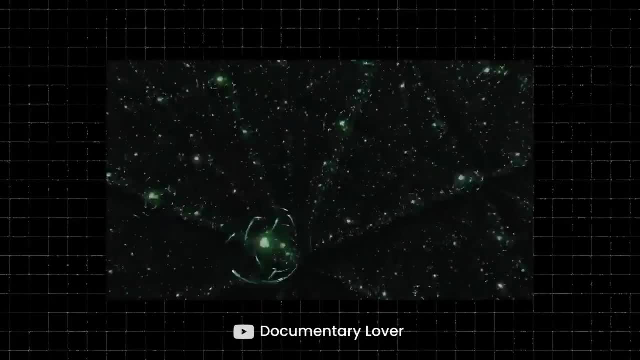 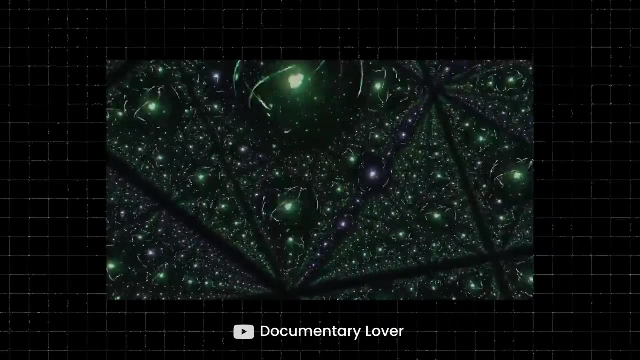 version called M-theory, proposed in 1995 by the physicist Edward Witten. The scientist believed that the different variations were all just different manifestations of a single underlying theory because, according to research, certain forms of mathematical transformations could be used between these versions. Put simply, it's possible all these theories are. 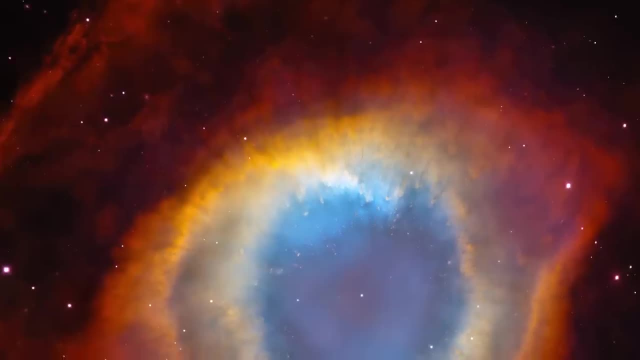 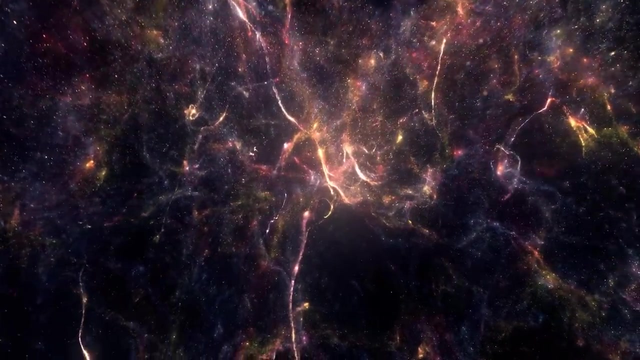 just different ways of mathematically expressing the same idea. But while M-theory remains the leading candidate for the theory of everything, much more advanced mathematical tools need to be invented to fully understand it. So far, string theory is very speculative and nearly impossible to test explicitly. The theory of the M-theory 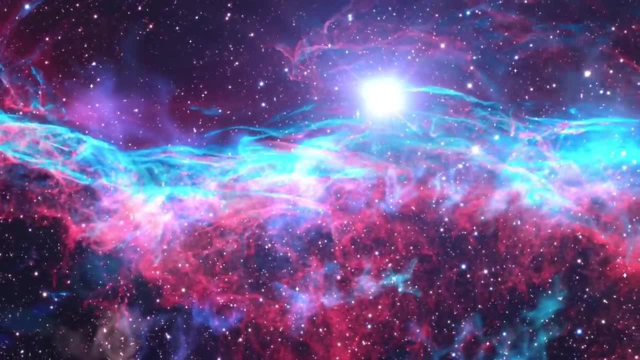 is the only theory in the world that can be used to fully understand it. The theory of the M-theory is the only theory in the world to test experimentally. But just because it's difficult to prove doesn't mean the theory is wrong. 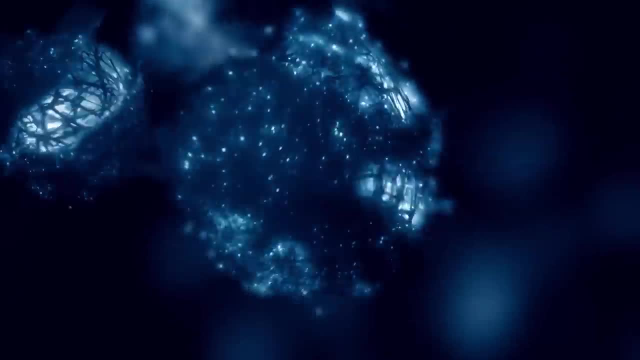 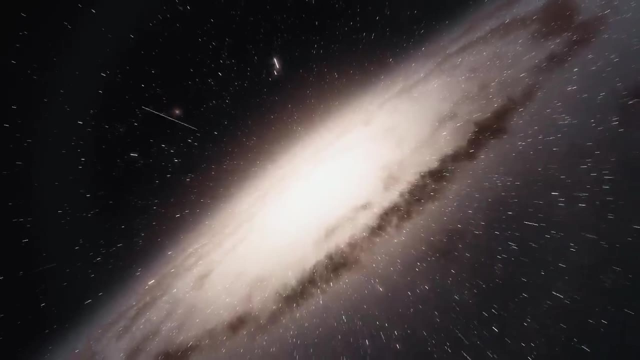 Einstein once said there was not the slightest indication that nuclear energy would ever be obtainable, as it would mean shattering atoms at will. And here we are, using nuclear power plants on a daily basis. Do you think string theory is our best shot at explaining? 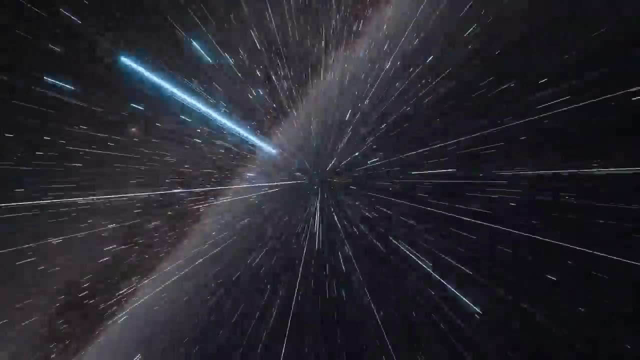 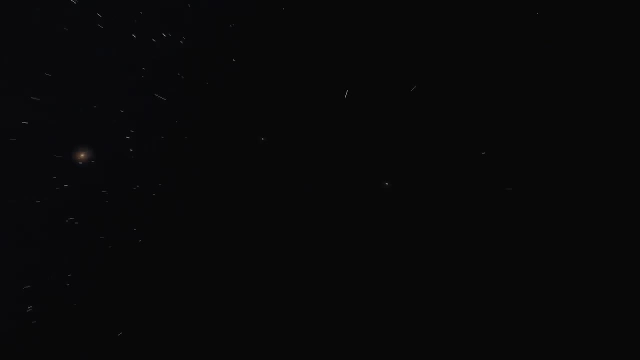 the universe and will it ever be proven? Sound off in the comments and thanks for watching. I'll see you in the next video.